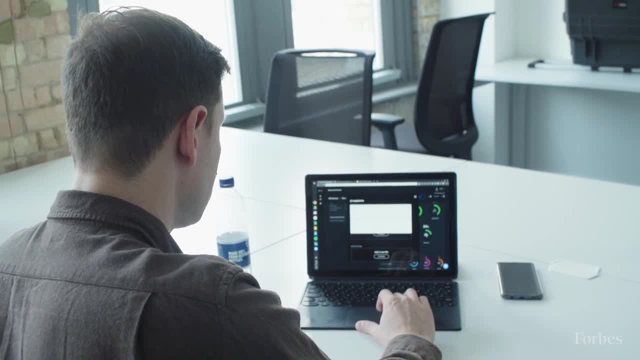 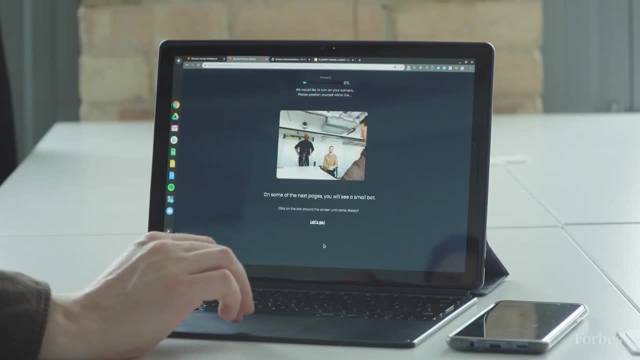 change for consumers. So one of the things that we look at here is: let's see if Tim Hortons is disgusting, Our competitor is going to be McDonald's. We need people to look at this. So we're plugged into a bunch of globally sourced panel providers. Now we're 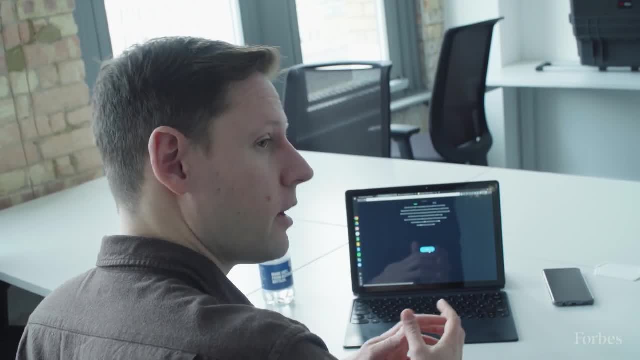 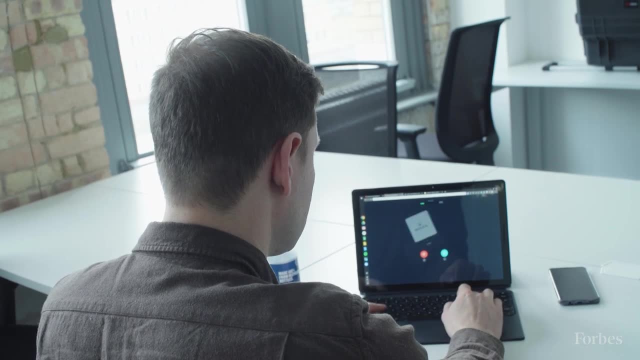 going to enter something we call memory tests. So this is one of our first subconscious measurements. We call it Tinder for brands. Is Rolex cheap? Do I disagree or agree with the statement? So I disagree with that statement. So what we're doing here is we're building a bank. 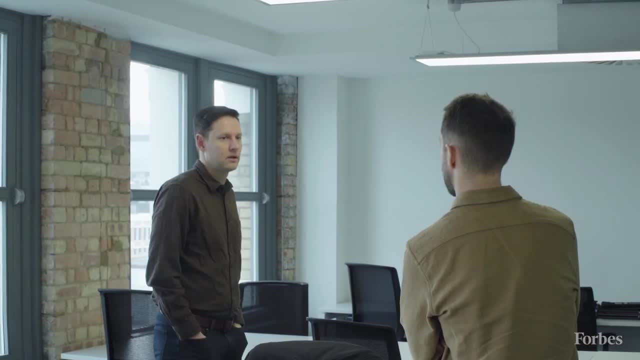 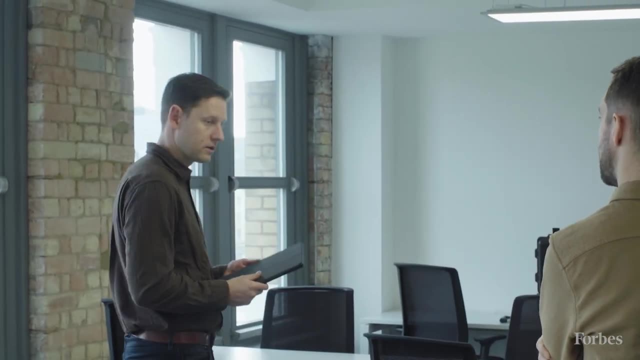 of my reaction times. He says that, aside from assisting publishers, he sees all kinds of uses for his technology. It might, for instance, be used to detect when a crowd is about to riot. I think, yes, it will go in that direction, Those types of public protection principles. 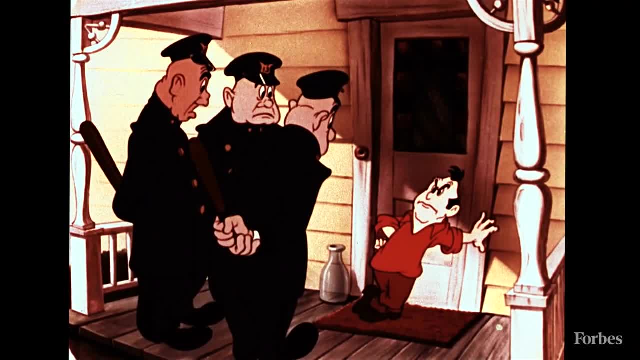 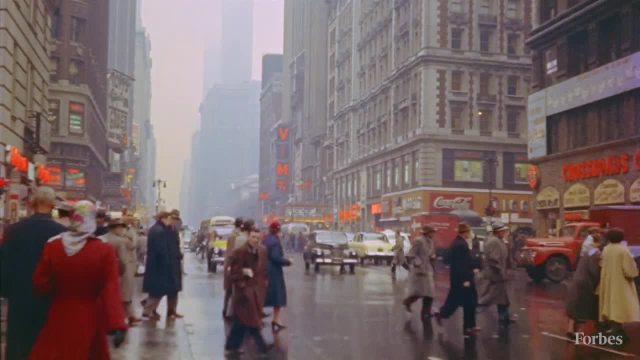 to help for? can we identify a crowd that's about to turn into a riot? Can we tell somebody who's really nervous Even forget? just public protection, but more transport safety, Just people who are moving through the city? Is there a particular crosswalk that actually? 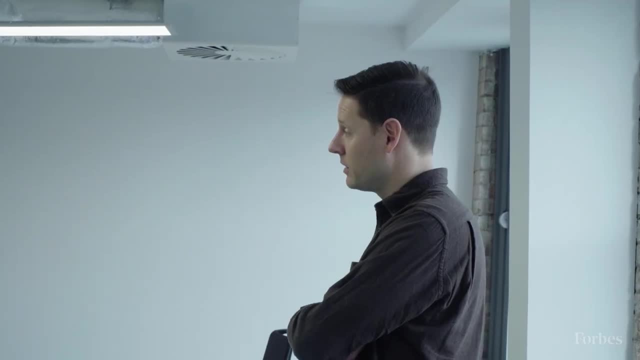 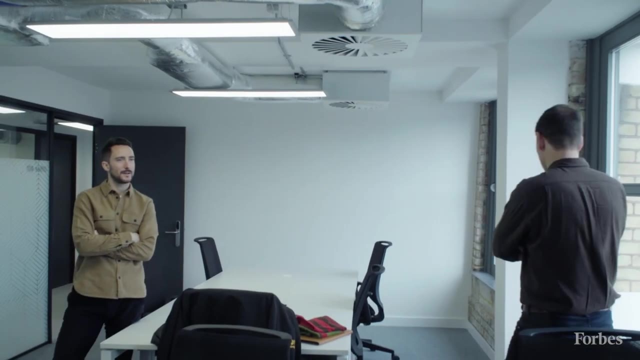 people almost get hit all the time. We just need to adjust the light length. But ethics are important to ethics. It's important that anyone entering this new market says Selizak. His company has already decided it won't be working with certain people out of those ethical concerns, namely 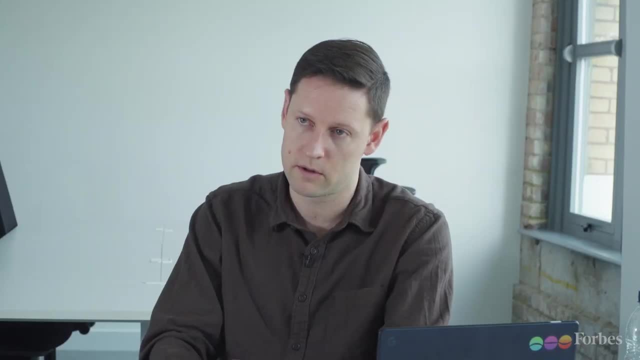 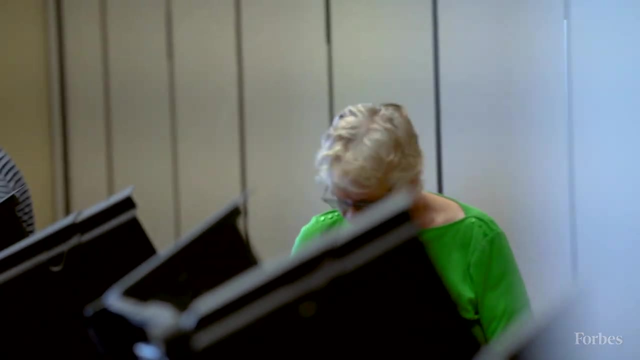 gambling companies and politicians. When we work with our customers, we have in our contracts that our first and primary obligation is to the data owner, And the data owner in our case is always the individual. So we stand firmly on the side of the voters versus the politicians. 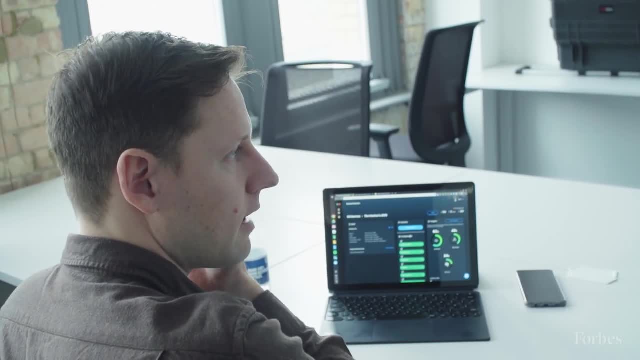 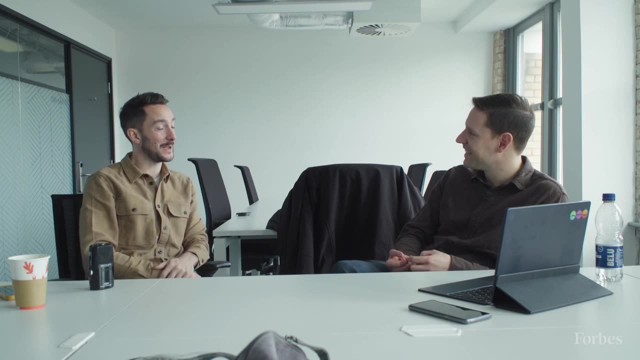 In the end, Selizak thinks that, rather than dehumanize us emotion detection, AI will actually become more human. He thinks that where people are loaded with personal baggage when they try to determine others' feelings, AI can make better, more objective determinations. 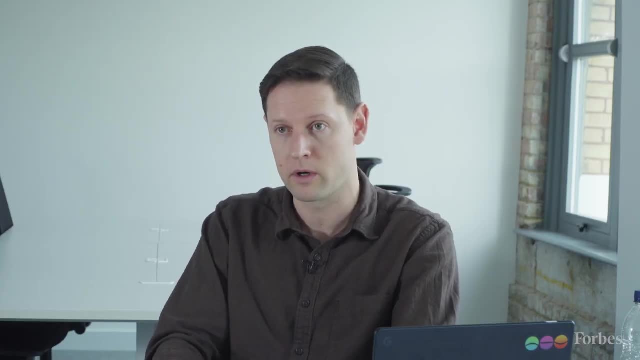 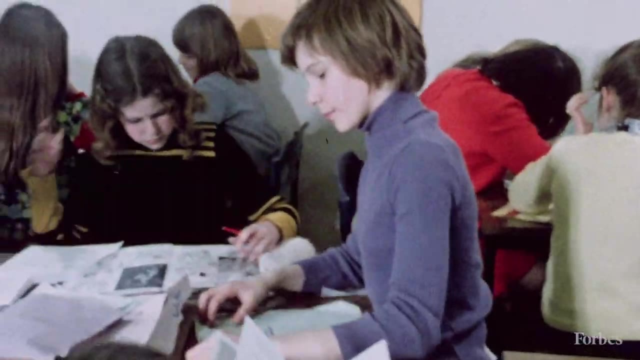 I have a talking series coming up this year which is: AI will actually make us more human. It will only do so if we bring non-engineers and artificial intelligence people along for the ride. So you have to bring everybody. It has to be a collective global movement.